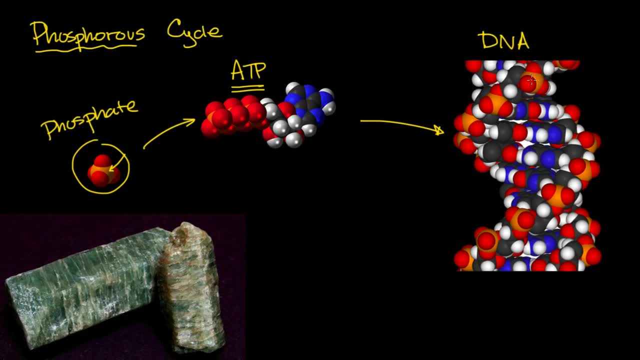 because life as we know it involves ATP and involves DNA and many, many other things that phosphates are involved with. Now phosphate, or phosphorus, I should say, in particular, is a little bit different than carbon or nitrogen in that it's not found in the atmosphere. 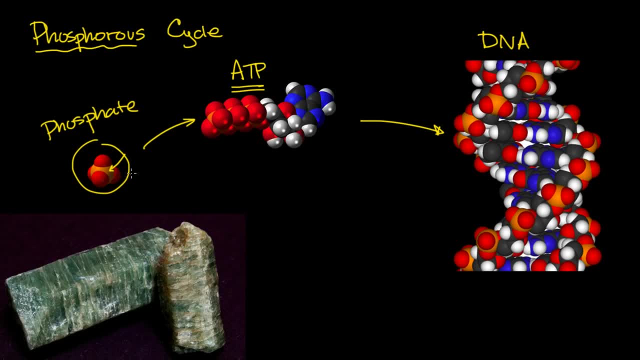 It's not typically found as a gas. Instead, phosphate is going to be formed, is going to be found in rocks, And it's going to be phosphate-based rocks. There will be other elements in there. It could be chlorine, it could be. 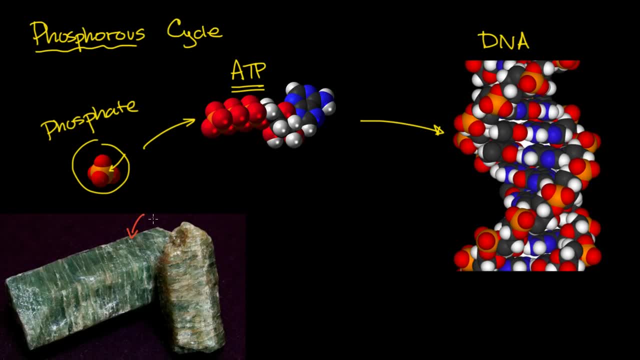 well, there's a bunch of different types of phosphate rocks, But when they're in their sedimentary form, so let me create some soil here. So let's say this is, let's say this is. let's say this is, let's say this soil has some phosphates in it. 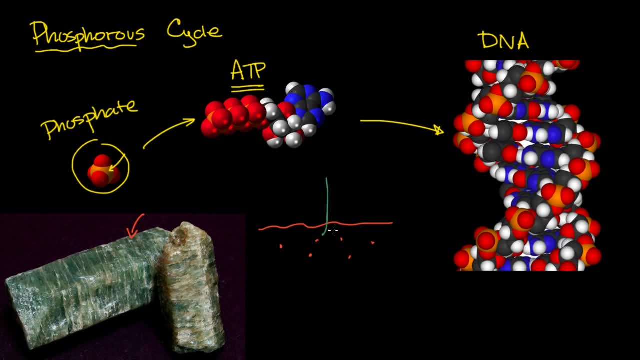 Well then, it allows things like plants to grow in that soil. So this is a plant growing in that soil And the plant- and we've talked about it before- it could be. it could be taking it's fixing carbon from the atmosphere using light energy. 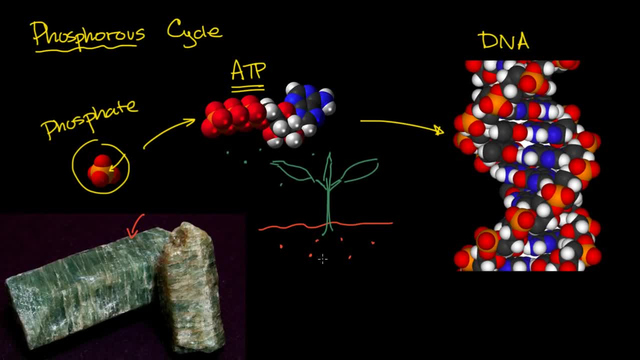 But its phosphate is going to come from the soil. That phosphate was already there and that helps that plant grow, because that plant needs that phosphate For its ATP, its DNA, its RNA and for other things, And phosphate is often considered a rate-limiting factor. 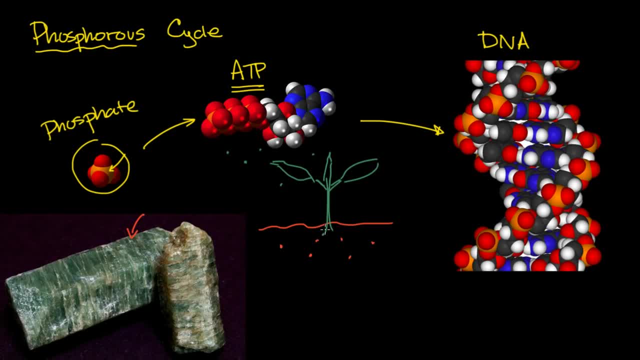 for the growth of things like plants, And that's why a lot of fertilizers will have- will have- phosphorous in them, or phosphates or will, and nitrogen's another one. So next time you think about fertilizer, you're fertilizing things in your garden. 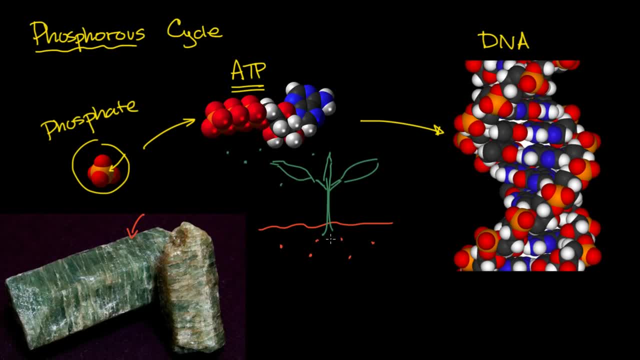 look at the ingredients, You will see phosphate there, because that might be the scarce resource or the thing that is limiting the actual growth of the plant. And then you might say: well, I have ATP and DNA in my body. How do I get phosphates? 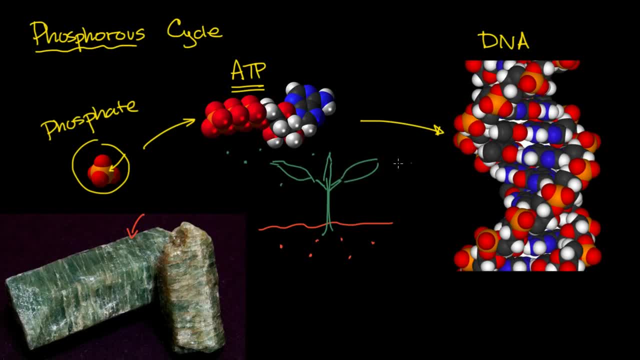 Well, you get it by eating plants. So this is this, is you eating a plant? So the plant goes back there. And how? how does this form a cycle? Well, when any of this living matter dies- and I've said in previous video, 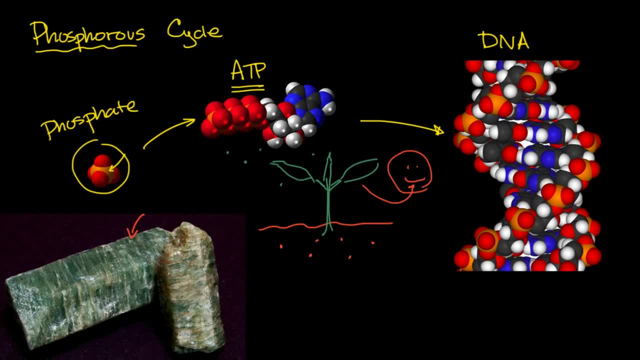 I'll show the dead plant, because a dead animal is. it's just a little darker. So whenever you see so this is a plant, now it's dead, Let's say it got buried somehow Some soil, so it's all.